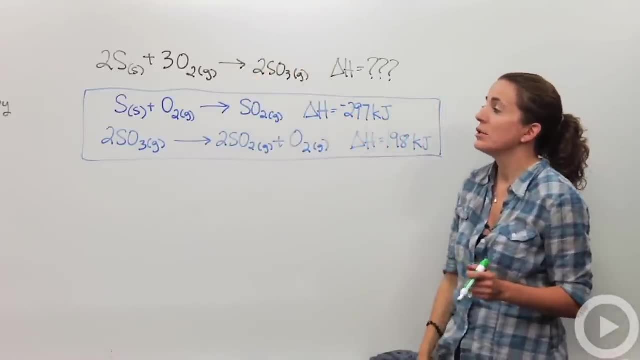 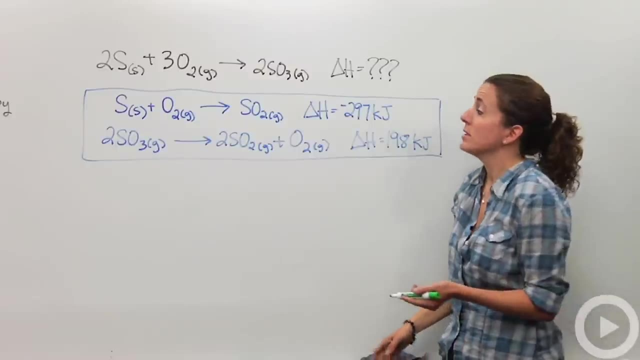 and that way I can figure out my delta H if I add up the two H's. So first I have to make sure that I have these reactions actually do add up to the final reaction. So let's look at this first thing. I need two sulfurs on my reactant side. 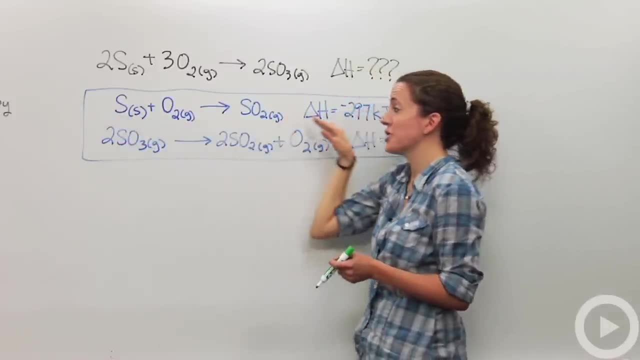 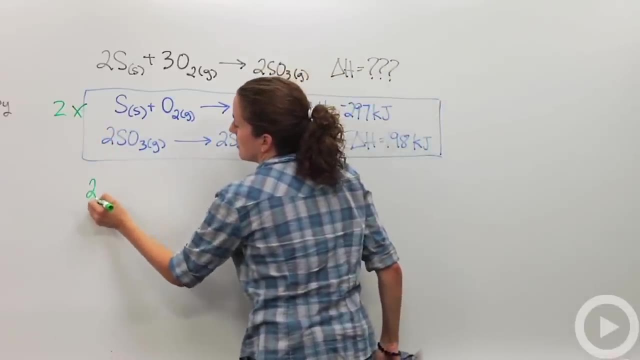 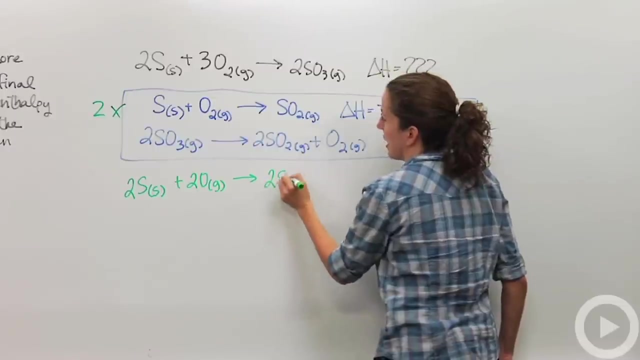 Well, here's sulfur, but I only have one, So I'm going to multiply this whole reaction by two so I can get two sulfurs on my reactant side. So I'm going to multiply this by two, So that makes two sulfur plus two oxygen gases yields me two sulfur dioxides. 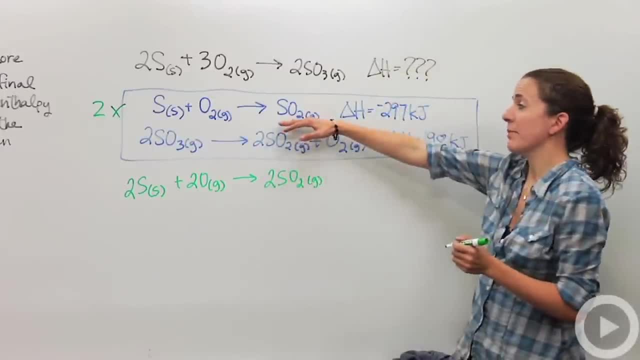 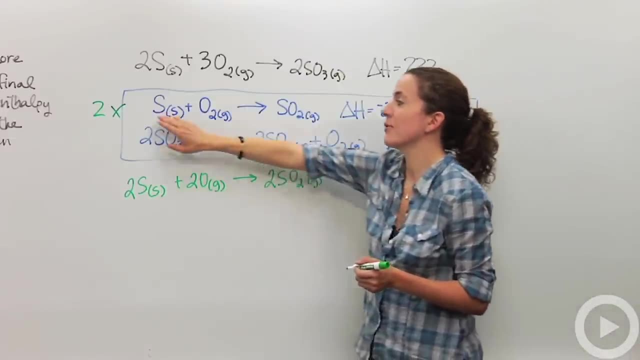 And because I multiplied the reaction by two. this also must be multiplied by two Because this negative 297 kilojoules is telling me how much energy is going to be released for one mole of sulfur, But I'm now doing two moles of sulfur. 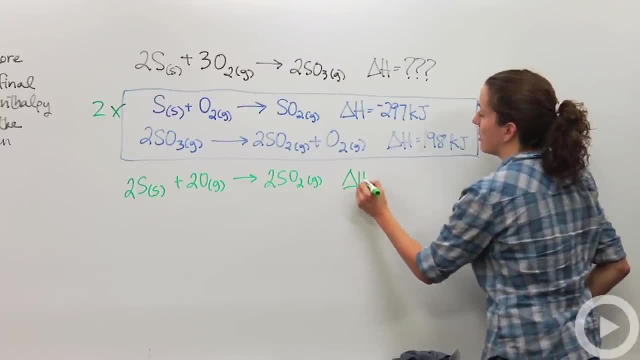 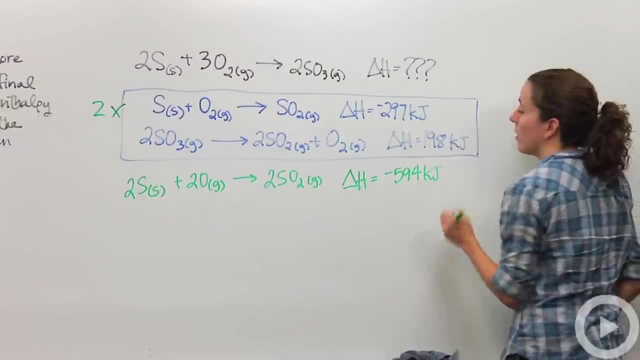 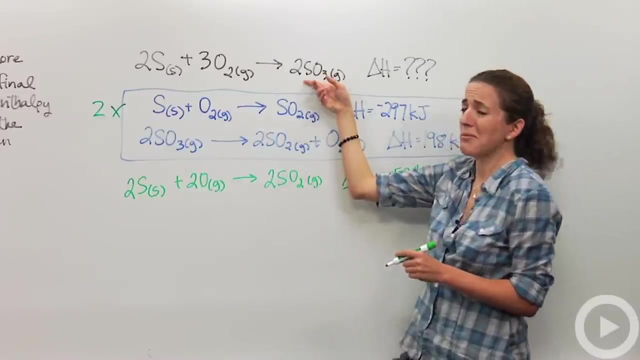 So I'm going to multiply this by two, So my delta H is now going to be negative 594 kilojoules. Okay, great. So now I have my two moles of sulfur on my reactant side. That's awesome. But now I have sulfur dioxide on my product side, and I don't want it. 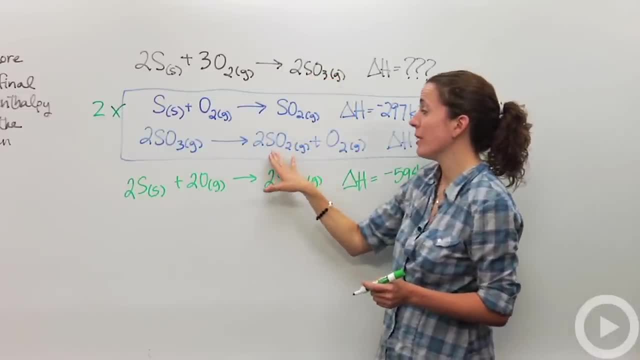 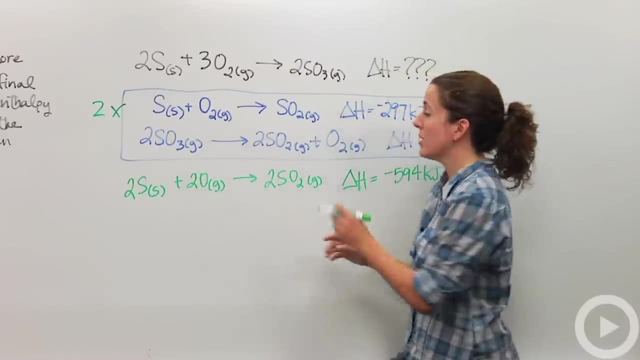 I want sulfur trioxide. So I'm going to look at this reaction here. Well, here's sulfur dioxide on the product side and sulfur trioxide on the reactant side. So I actually want to flip those around, So I'm going to do the reverse reaction. 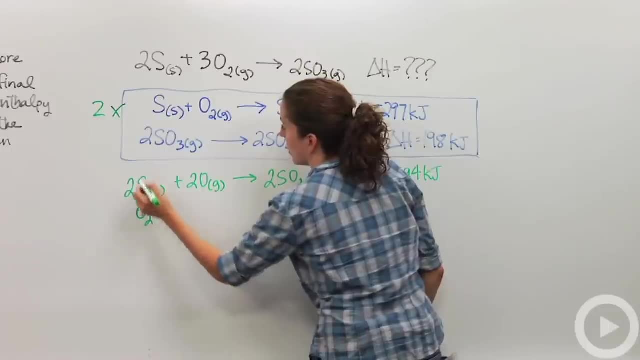 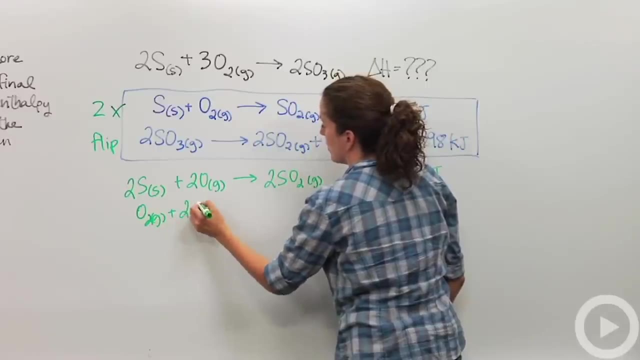 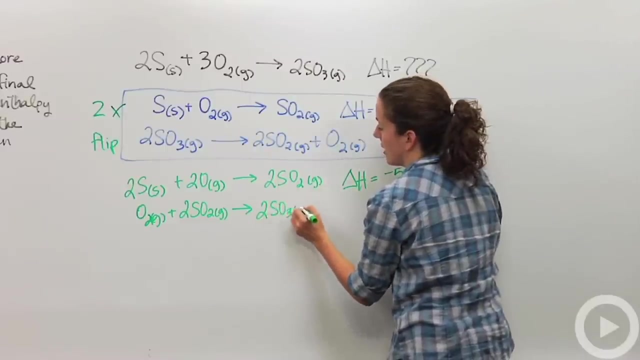 So I'm going to say oxygen gas. I'm going to make sure I note that Oxygen gas plus two moles of sulfur dioxide gas is going to give me two moles of sulfur trioxide gas. Okay, And because I flipped it, 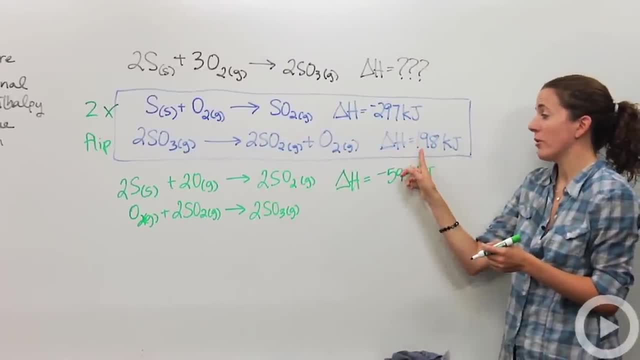 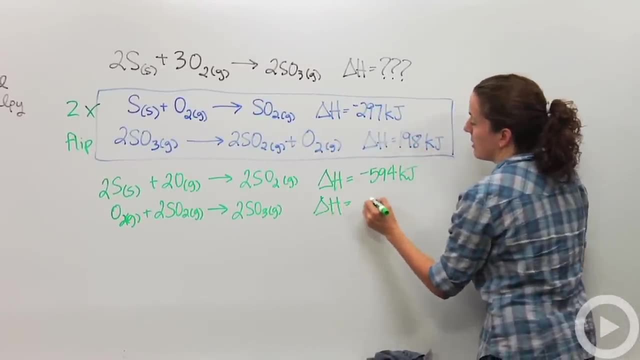 this, going this forward direction- is going to be an endothermic reaction. But if I reverse it- I'm going to- this is going to be an exothermic reaction. So this is going to be negative. So my delta H is going to be negative: 198 kilojoules. 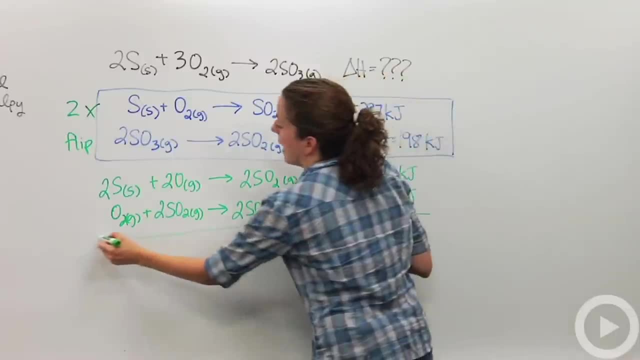 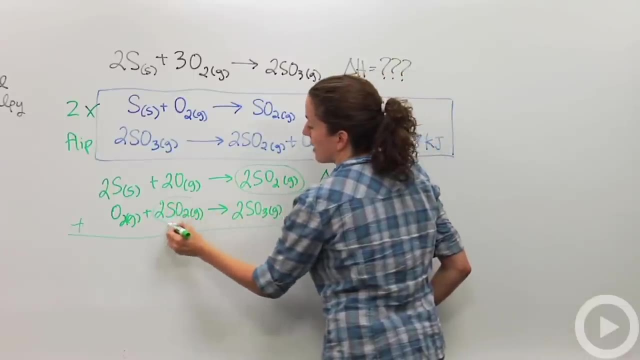 Okay, So let's make sure this works. So if I were to add these two reactions together, I note that I have two moles of sulfur dioxide here and two moles of sulfur dioxide here- I can cross those out because this is a product and this is a reactant, so I can just cross those out. 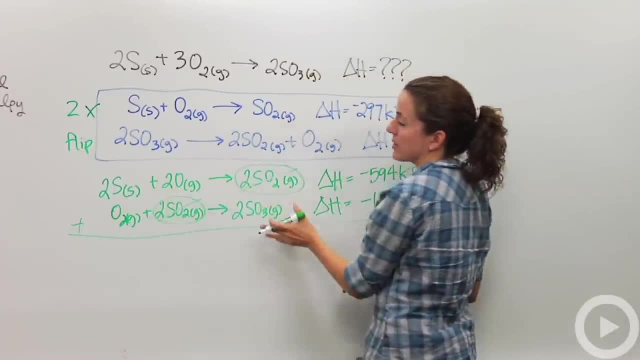 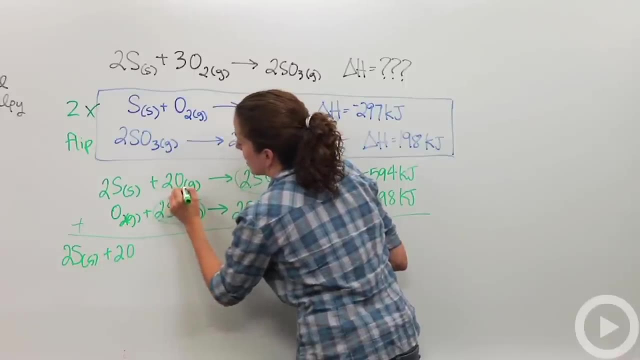 Okay, And now if I add everything up, I can't. I can't do anything else. I'm going to add everything up. So I have two moles of sulfur solid plus two moles of oxygen. This should be oxygen two. 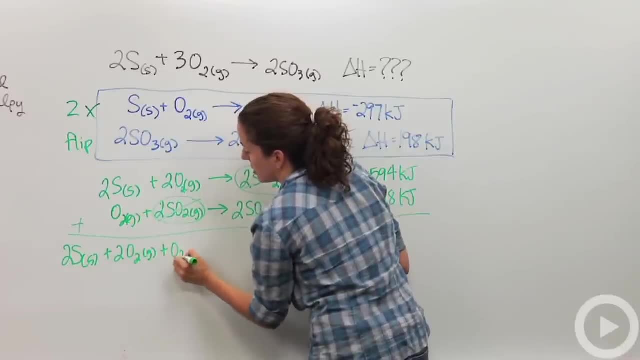 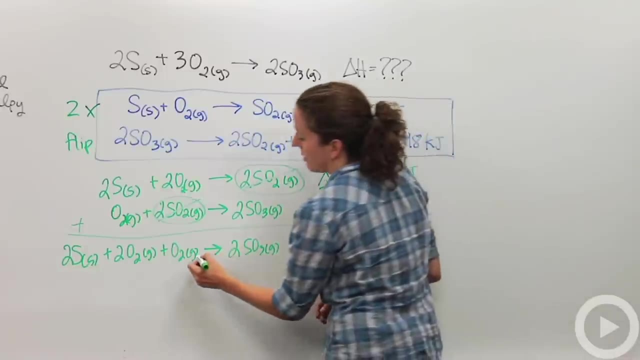 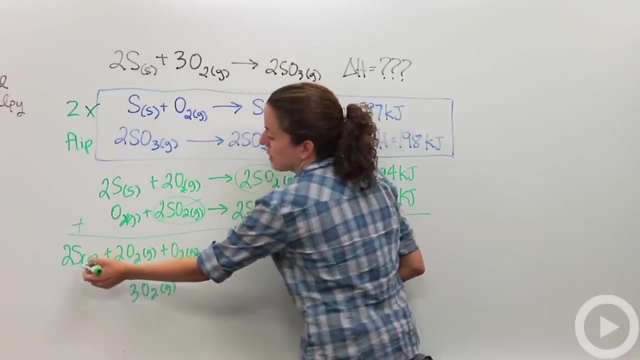 Sorry. O2 gas plus another mole of O2 gas yields two moles of SO3 gas. Okay, So what if I add these together? Two plus one is three, So I can say three moles of oxygen gas. So two sulfur atoms are. 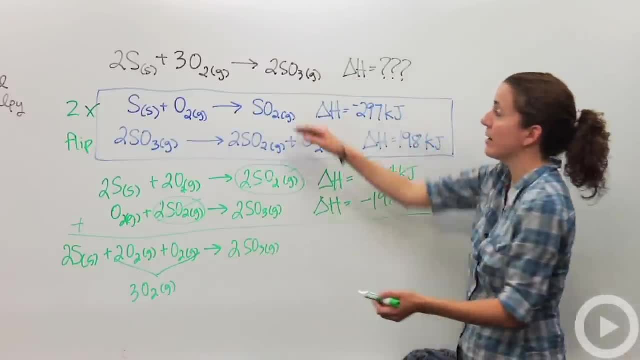 two moles of sulfur plus three moles of oxygen yields two moles of sulfur trioxide, Which is exactly what my original equation is. So, yes, I did this properly. I can check it off, And so I want to find my delta H. 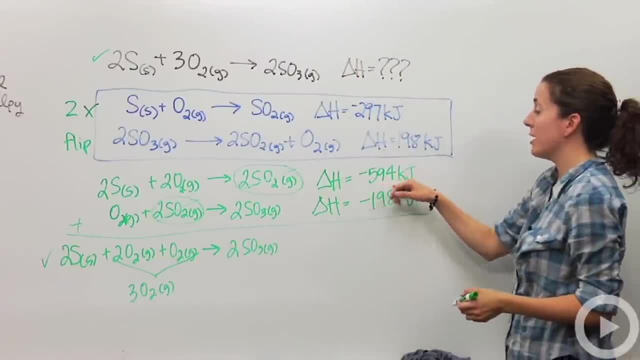 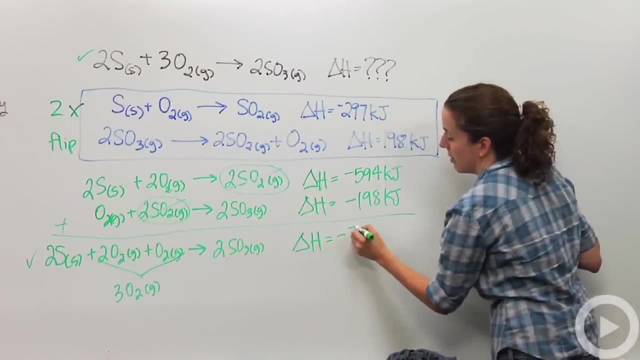 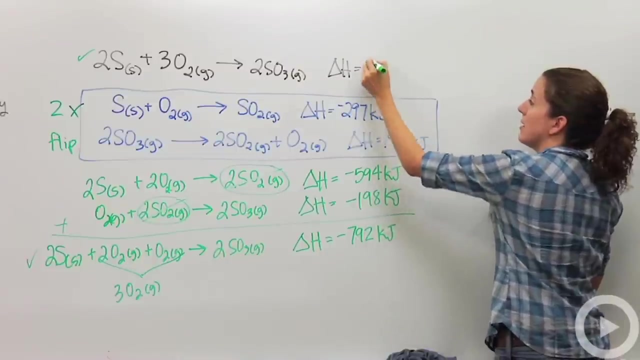 I'm just going to add these guys up. So negative 594 plus negative 198 is going to give me negative 792.. So negative 792 kilojoules, So that actually now I could know that this is negative 792 kilojoules because Hess's law says that I can do this. 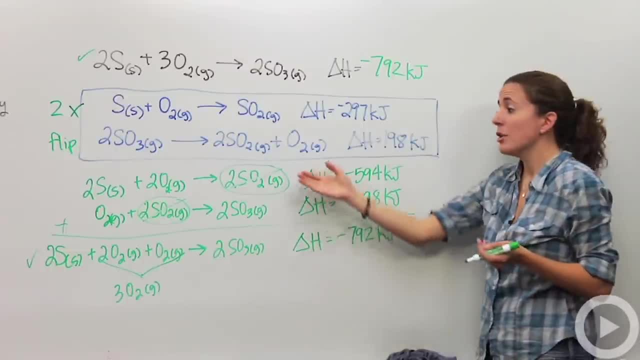 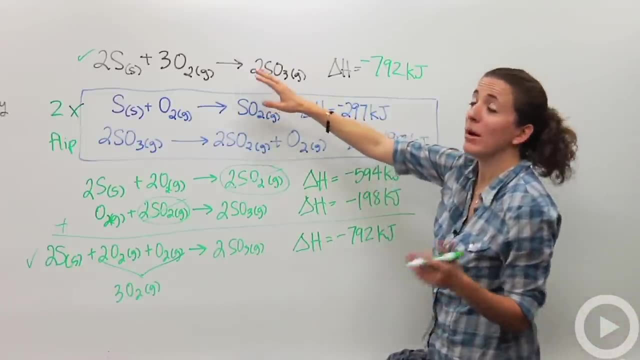 Okay, So this is basically Hess's law in a nutshell. You might have several different reactions, you're going to have to manipulate, But actually, once you get the hang of it, it's actually kind of fun and pretty easy. But I'm also going to do one last thing. 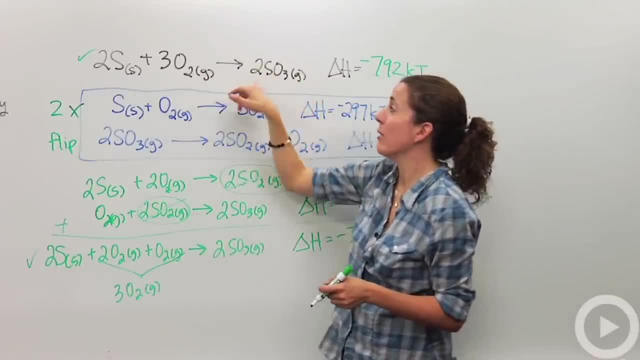 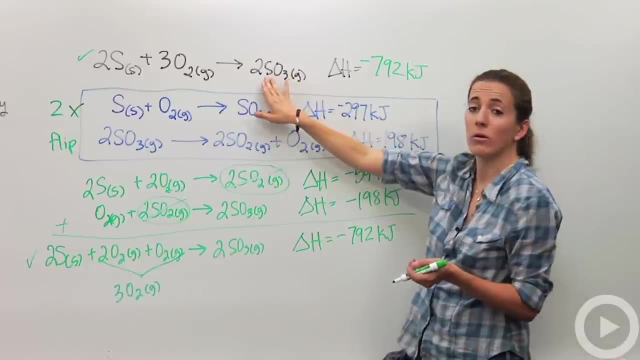 This is a reaction. It is a formation reaction, Meaning we're taking, we're forming sulfur trioxide from its elements. So, in order to do formation reactions, the best way is we want to get this to be one mole, So I'm going to divide the whole thing by two. 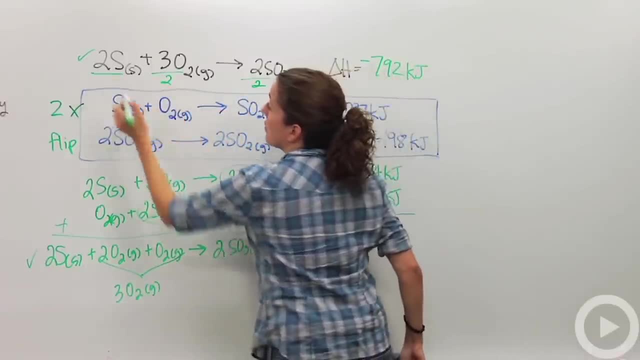 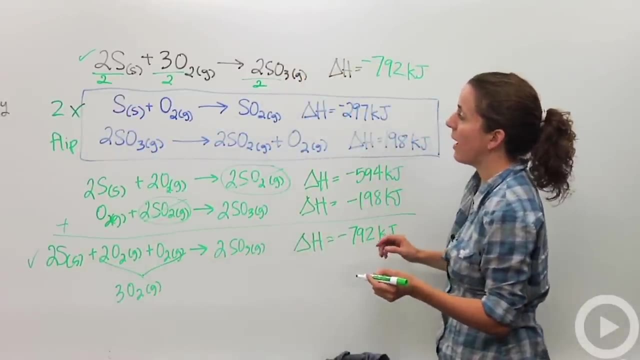 Because I don't like in formation reactions. if you want to learn more about them, there's a video. There's a video on that as well. But formation reactions have one mole of the product, So we're dividing everything by two. 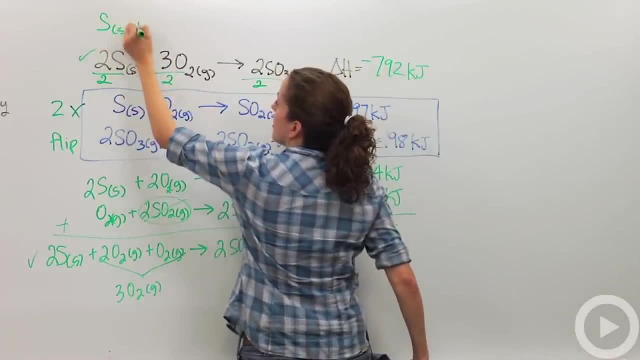 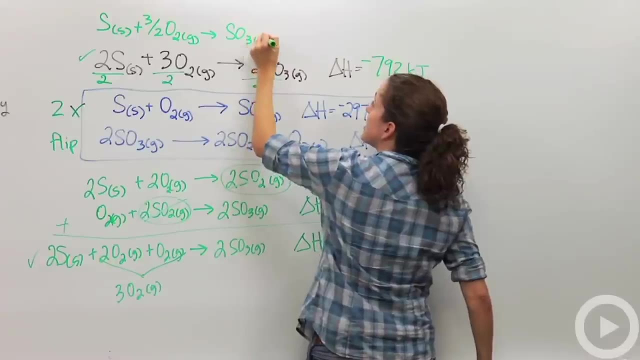 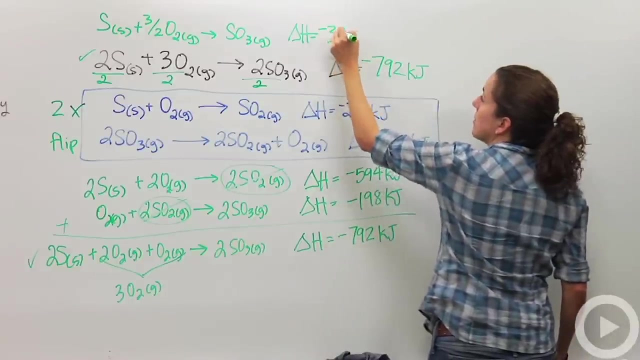 Which ends up with sulfur solid, plus three halves oxygen gas yields sulfur trioxide gas. And then my delta H is also going to be divided by two, Oops, Which is going to be negative 396 kilojoules, And we can actually say kilojoules per mole.